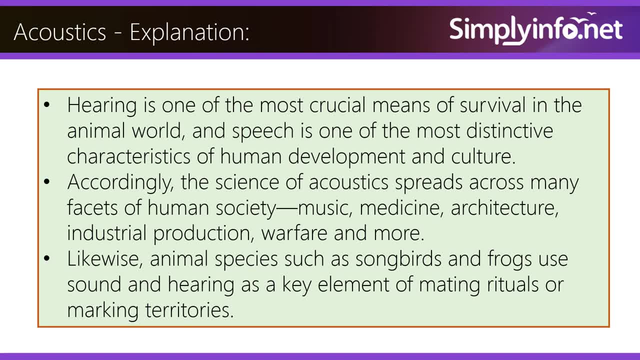 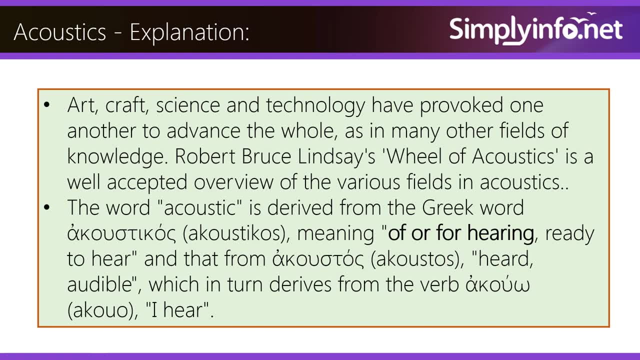 The use of human in crime. 4. The access to intellectual property to science. 5. The use of human worlds pass sunlight or water in the environment. knowledge, robert bruce lindsay. we love acoustics- is a well accepted overview of the various fields. 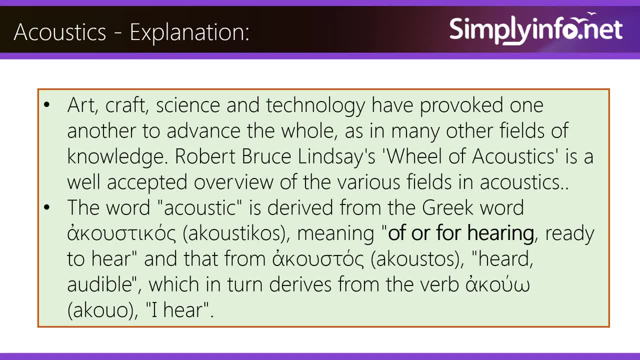 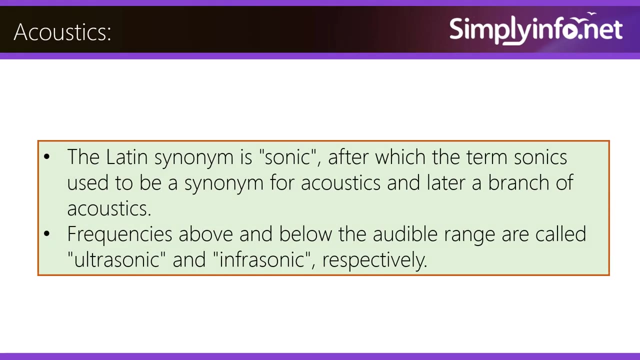 in acoustics. the word acoustic is derived from the greek word acousticos, meaning off, or for hearing, ready to hear, and that from acoustos, heard, audible, which in turn derives from the verb aquo. i hear the latin synonymous sonic, after which the term sonics used to be a synonym for acoustics, and 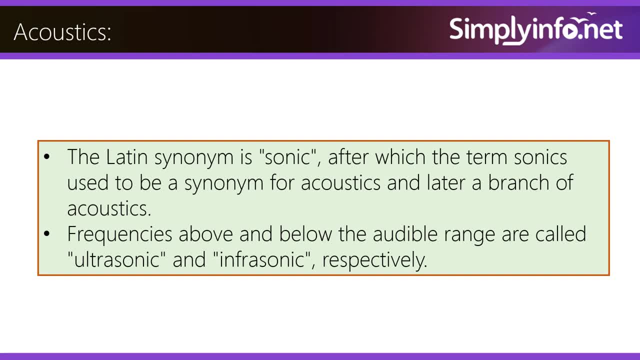 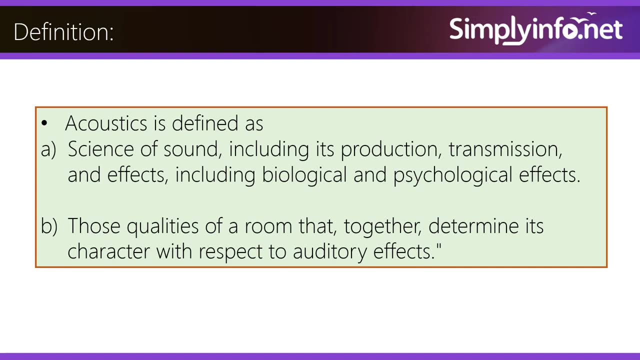 later a branch of acoustics. frequencies above and below the audible range are called ultrasonic or infrasonic respectively. definition: acoustic is defined as signs of sound, including its production, transmission and effects, including biological and psychological effects, Those qualities of a room that together determine its character with respect to auditory effects. 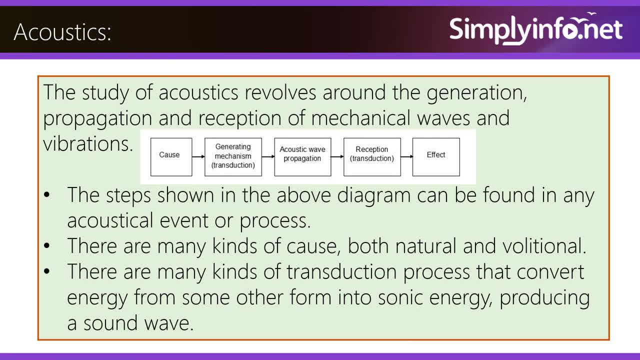 The study of acoustics revolves around the generation, propagation and reception of mechanical waves and vibration: cause, generating mechanism, transduction. acoustic wave propagation: reception, transduction effect. The steps shown in above diagram can be found in any acoustical event. 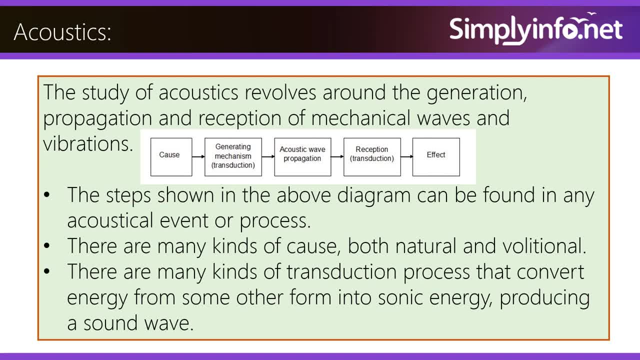 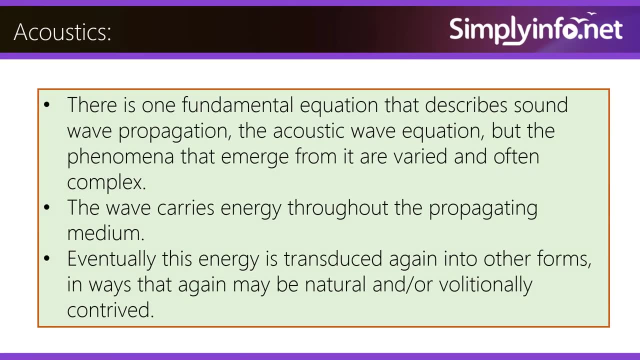 or process. There are many kinds of cause, both natural and volitional. There are many kinds of transduction process that convert energy from some other form into sonic energy. There is one fundamental equation that describes sound wave propagation, The acoustic wave equation. but the phenomena that emerge from 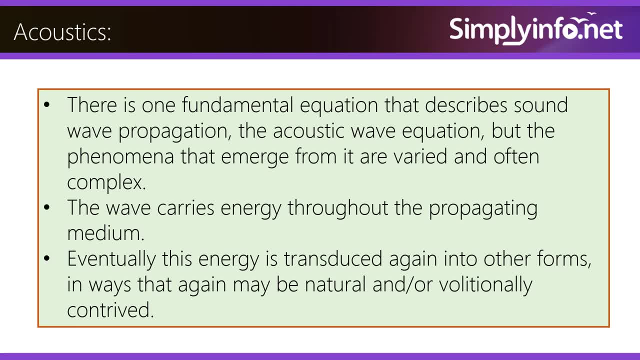 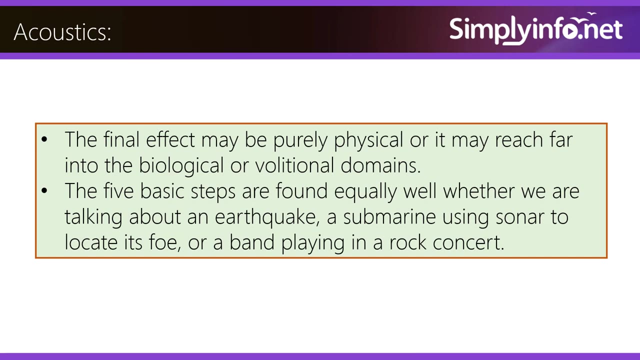 it are varied and often complex. The wave carries energy throughout the propagating medium. Eventually, this energy is transduced again into another forms in ways that again may be natural and unnatural. The final effect may be purely physical or it may reach far into the biological or volitional. 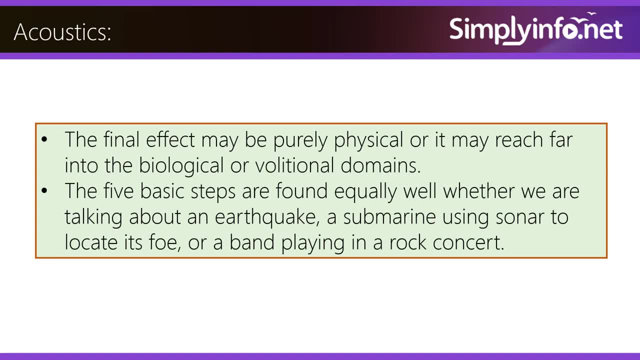 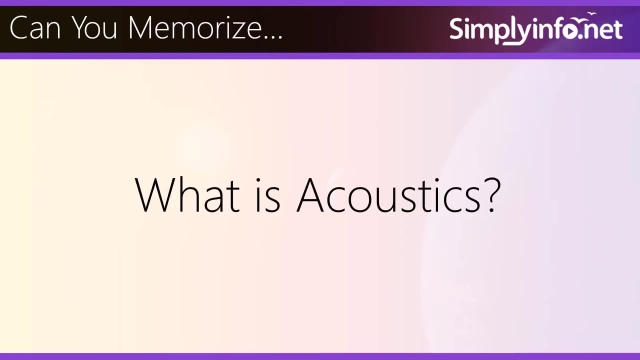 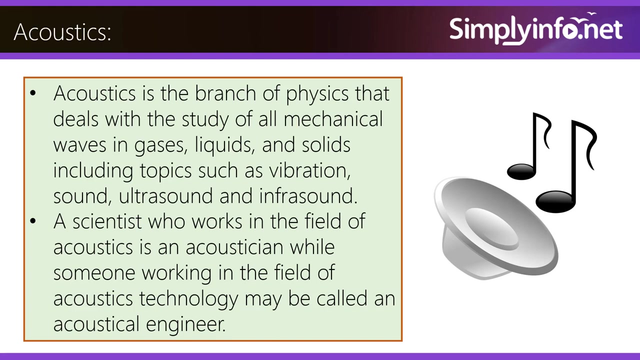 domains, The five basic steps are found equally well, whether we are talking about an earthquake, a submarine using sonar to locate its foe or a band playing in a rock concert. Can You Memorize What is Acoustics? Acoustics is the branch of physics that deals with the study of all mechanical waves in 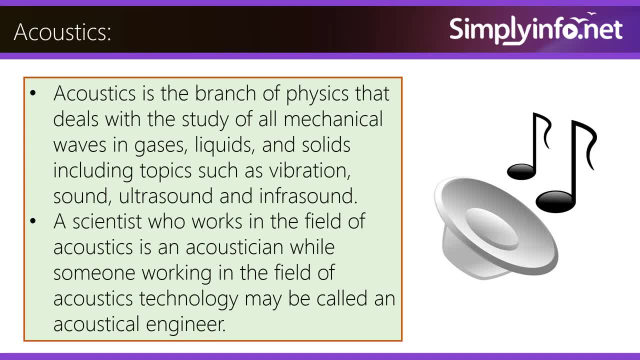 gases, liquids and solids, including topics such as vibration, sound, ultrasound and infrasound. A scientist who work in the field of acoustic is an acoustician, while someone working in the field of acoustic technology may be called an acoustical engineer. 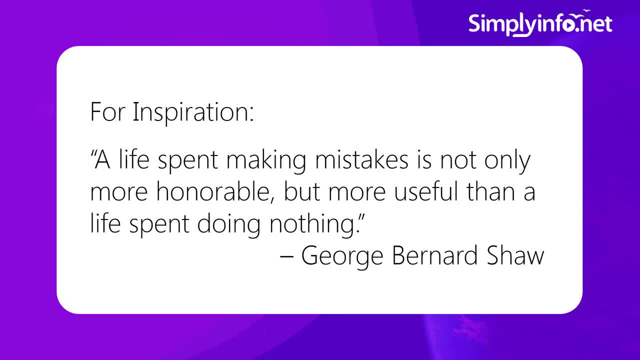 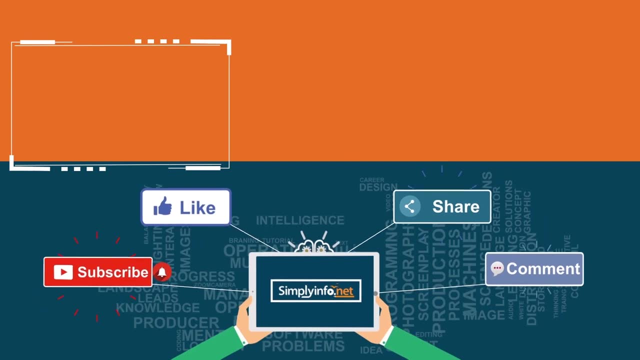 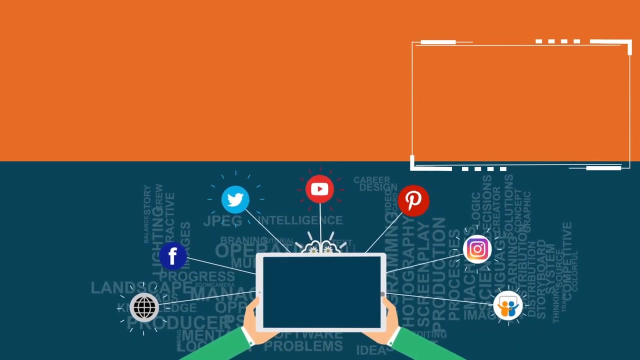 FOR INSPIRATION. A life spent making mistake is not only more honourable but more useful than a life spent doing nothing. George Bernard Shaw. Subtitles by the Amaraorg community.